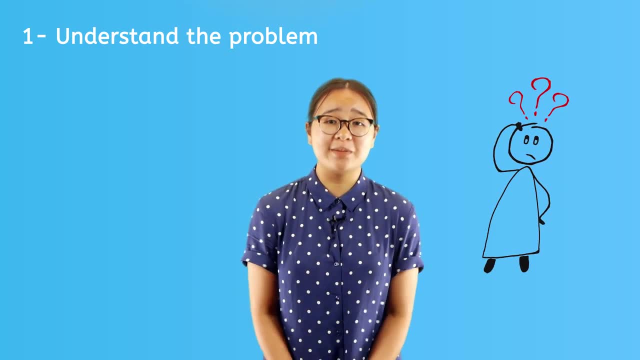 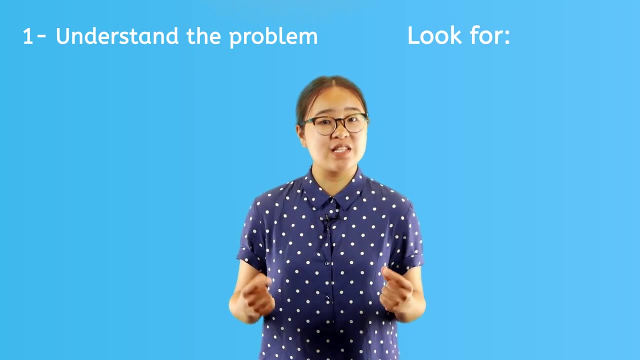 you're looking for, you'll get frustrated and want to give up. To understand a word problem. read it carefully once, then read it again, looking for important clues like keywords, examples and more. Write down the important numbers and, of course, the question the problem asks. 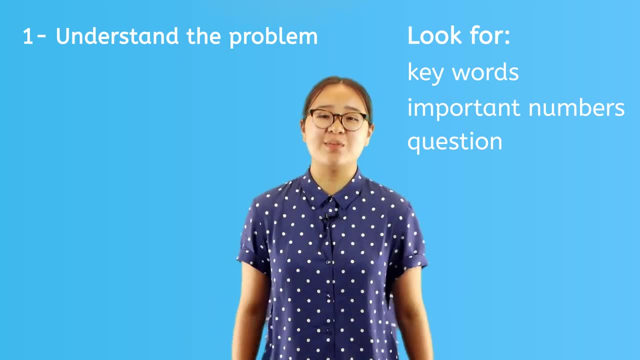 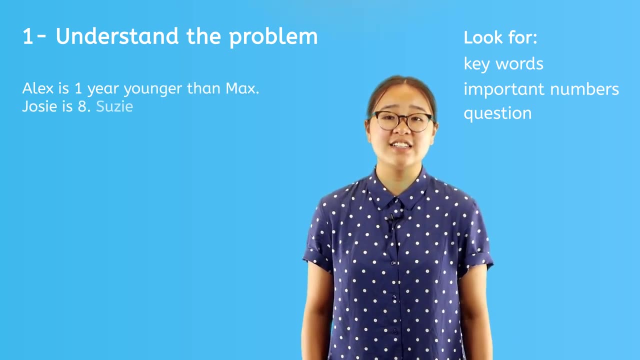 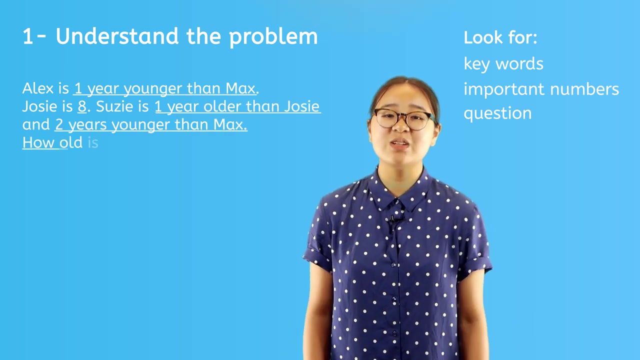 I like to underline or highlight important information. It's not just. Alex is one year younger than Max. Josie is eight. Susie is one year older than Josie and two years younger than Max. How old is Max Then? to be sure you fully understand it, reread the problem a third time. 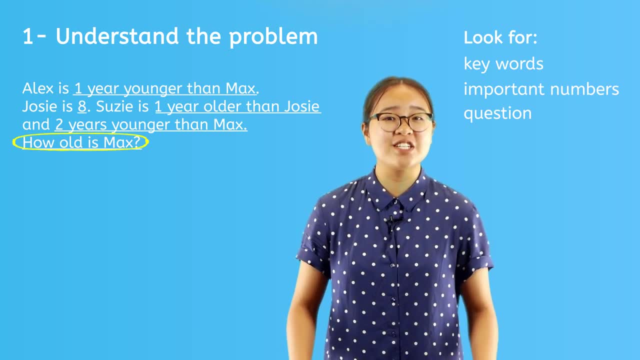 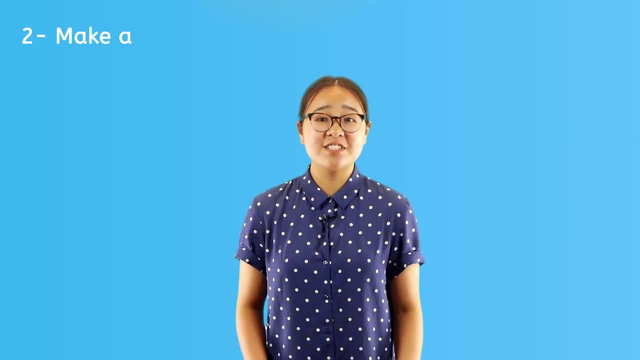 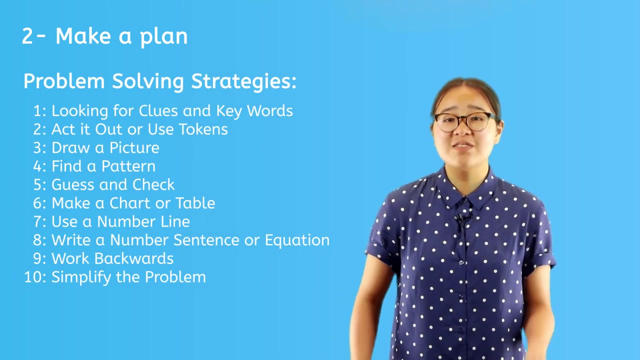 Before you tackle the problem, be sure you have understood the question very well. Once you've understood the problem, it's time to make a plan to solve it. First, you will choose one of the several problem-solving strategies. To learn some problem-solving strategies from our site, watch the videos labeled Problem-Solving Strategies. 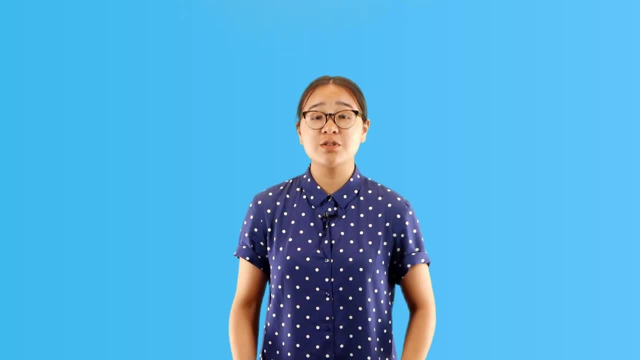 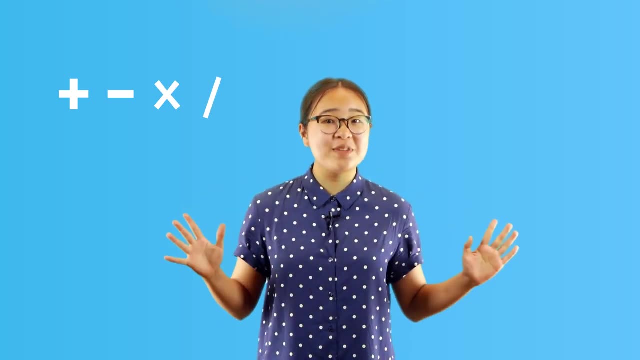 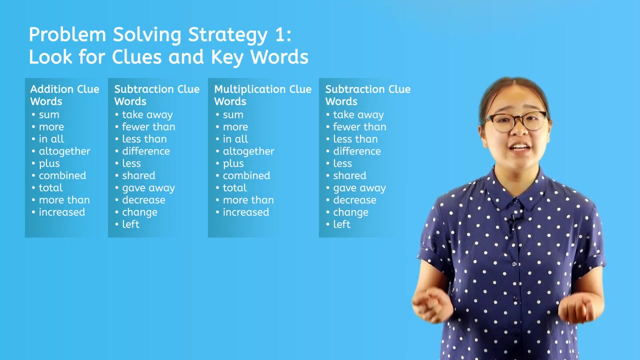 Once you have chosen an appropriate strategy, reread the question and ask yourself if you'll need to add, subtract, multiply, divide or a combination of these. In Problem-Solving Strategy, Video 1,, look for clues and keywords. You will find a list of clues to help you know which operations to use. 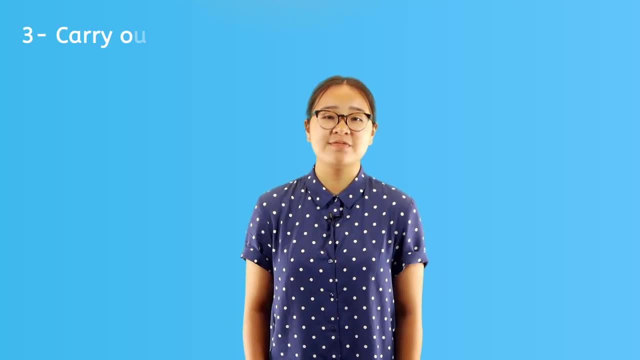 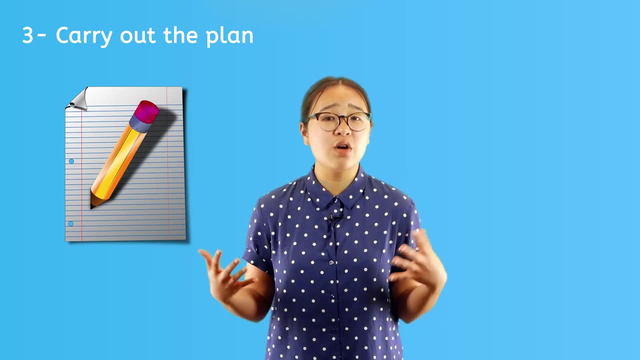 Now that you have a plan, you can work out the word problem. You can use a notebook or scrap paper to solve the problem. It's okay if it gets messy or if you have to start over a few times. That's what problem-solving is all about. 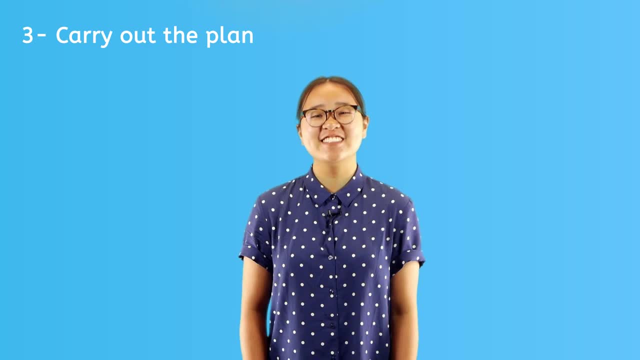 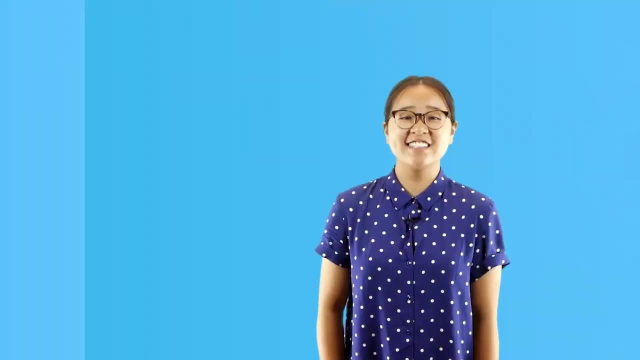 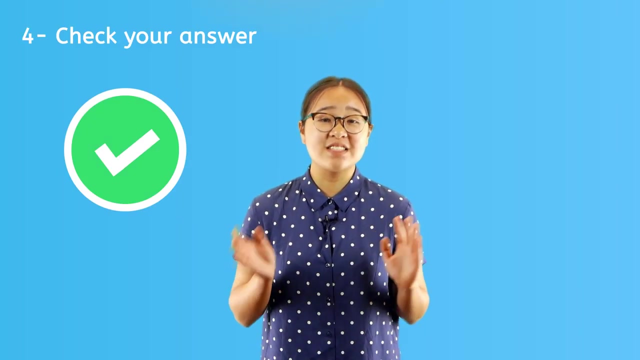 Just don't give up. Whenever you get stuck carrying out the plan, remember to always go back and reread the problem, And the final step to solving any word problem is to check your answer. Go back to the problem and see if your answer makes sense. 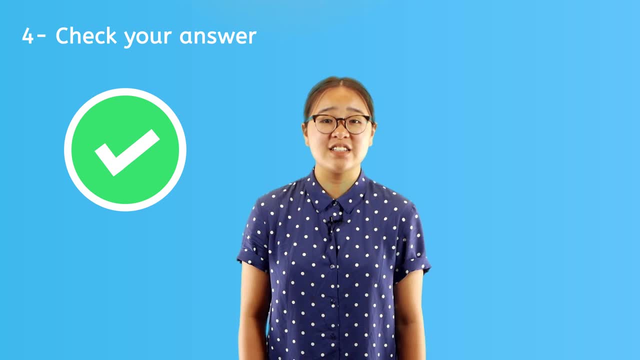 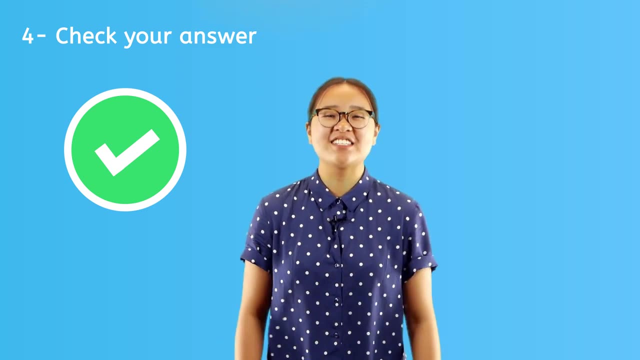 Is it reasonable? If it is, great. If it is not, you'll have to go back to Step 1 to make sure you've understood the problem correctly. Then check that you've calculated correctly. You now have a solid plan to help you solve math word problems.